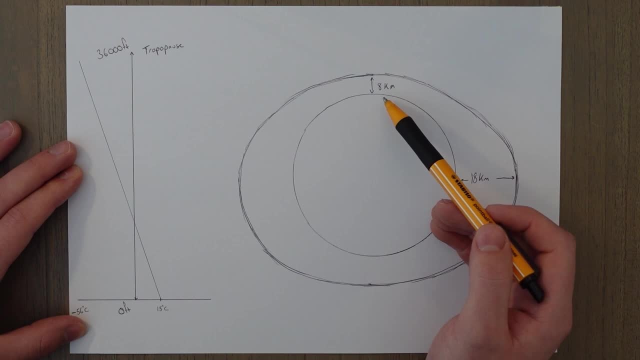 latitude. At the North Pole in the winter, for example, the air all compresses down and contracts, so the level of the tropopause can be down as low as 8 kilometers, and conversely, at the equator, in the summer the air expands out and the 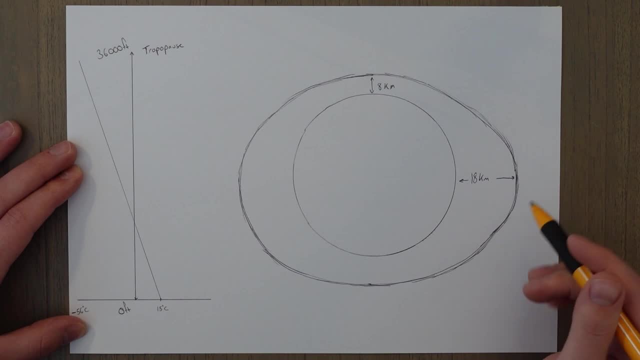 level of tropopause can expand up towards about 18 kilometers. We spend almost all of our lives in the troposphere, so it's where most of the weather occurs as well. It's where most the water vapor is, so it's the most important for us in terms of meteorology. The next level as we climb up is known: 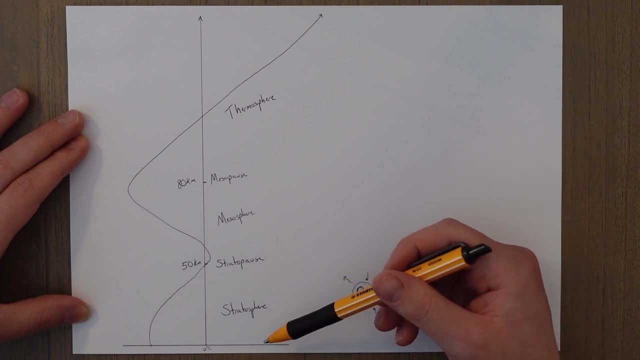 as the stratosphere, which extends from the tropopause up to around a 50 kilometer altitude. This layer is characterized by the stop in temperature reduction, and as we rise up through the stratosphere, the temperature can either be steady or steady, or it can actually increase. The reason for this is due to the presence of ozone. 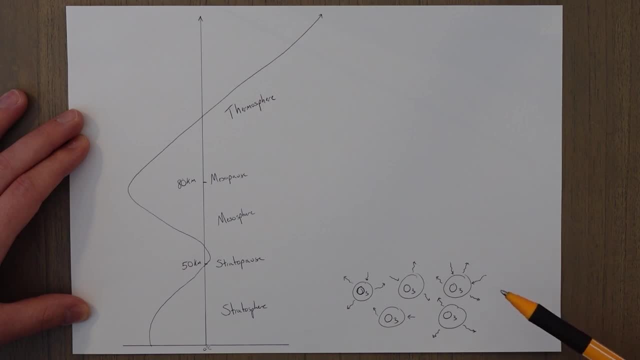 which is an oxygen-3 molecule, and this basically absorbs UV radiation from the Sun and it projects that heat out and heats up the surrounding air to the point where the temperature doesn't drop anymore and can actually heat up. The end point of the stratosphere is the stratopause and at this point the 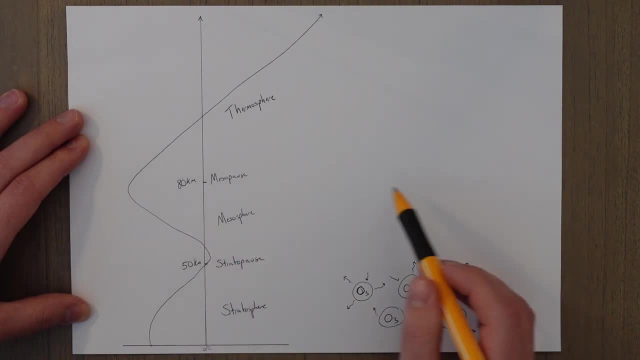 temperature starts again to reduce with altitude because there is no more ozone present. This continues to drop all the way down until the mesopause, which is located around 80 kilometers, and at this point we're in the final layer, which is known as the thermosphere, where 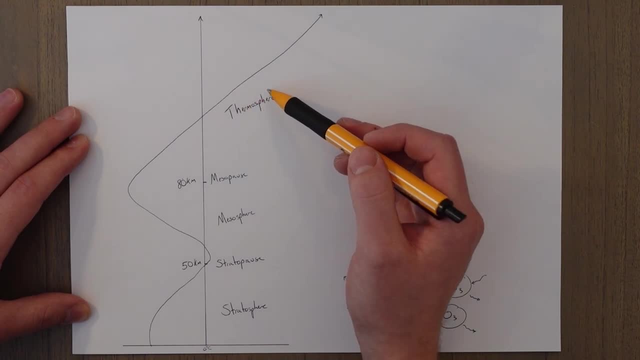 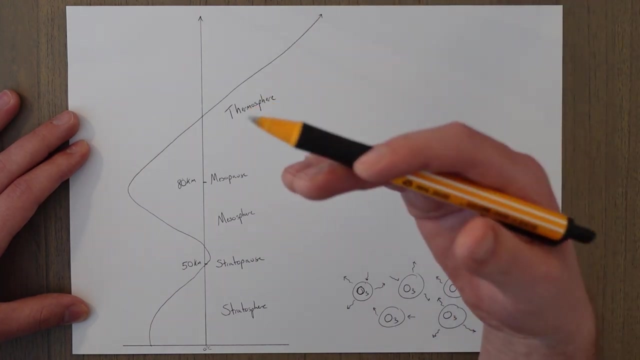 the temperature again starts to increase as we rise up the altitude levels. It's difficult to define an end point for the thermosphere because the outer most layer kind of blends into the surrounding space. There's no definitive line where there's suddenly an atmosphere. It's a very fluid sort of 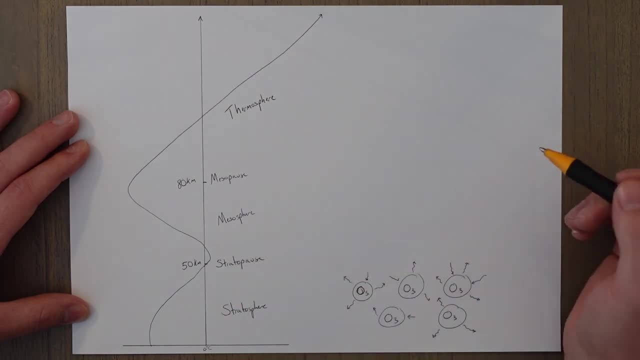 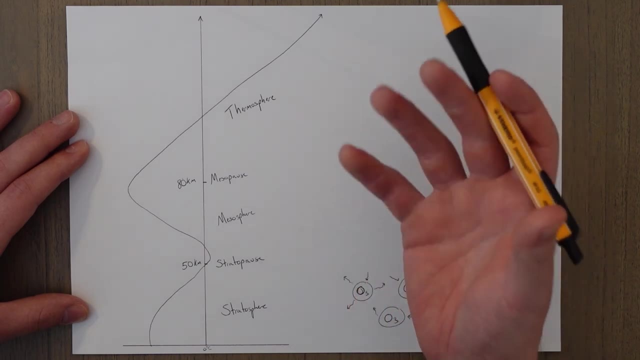 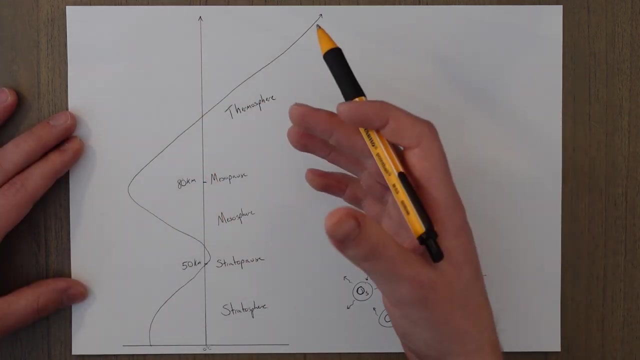 change from the space to our atmosphere. In the thermosphere we also have the ionosphere, which is very important for radio navigation. It's a layer which effectively bounces radio signals back down to Earth. This allows for radio signals to travel farther, but it's kind of more like a 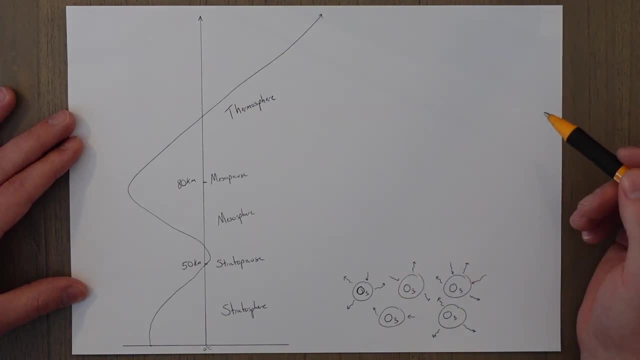 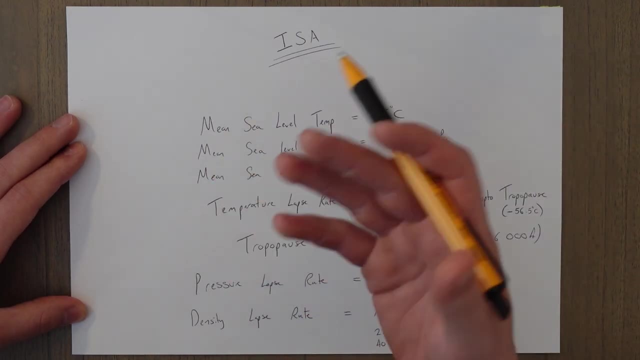 topic for radio navigation, not that important in meteorology. So because the atmosphere is constantly changing from day to day and depending on the time of year, all aspects of the atmosphere, such as temperature, pressure and density also change as well. So we use the international standard atmosphere for 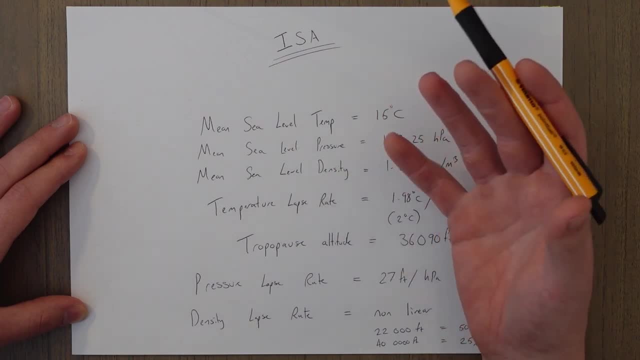 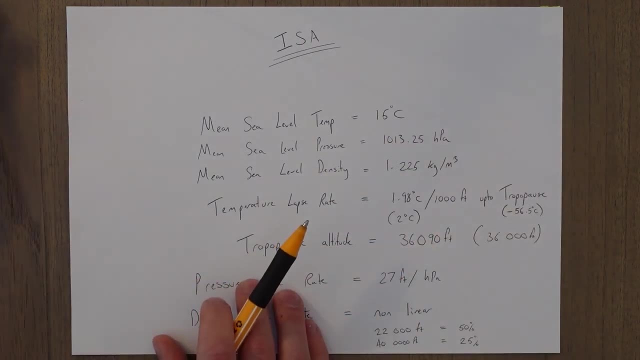 calculations and a baseline, and then we make small variations to this depending on the day's conditions, and it looks like this: There's a mean sea level temperature of 15 degrees Celsius. There's a mean sea level pressure of 1013.25 hectopascals. There's a mean sea level density of 1.225 kilograms per. meter cubed Temperature lapse rate is 1.98 degrees per thousand feet or 2 degrees per thousand feet, practically speaking up to the tropopause, and at the tropopause the temperature remains constant, minus 56.5 degrees Celsius. The tropopause is located at 36,090 feet or for practical purposes you can just say: 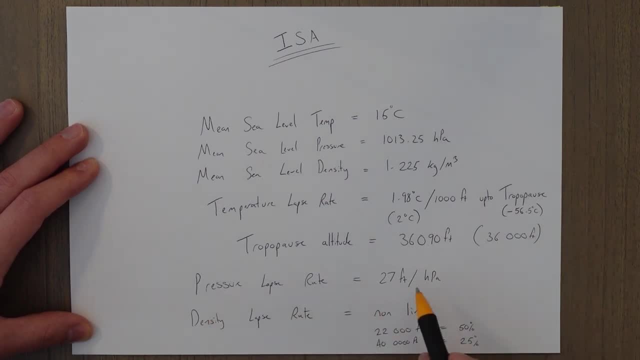 36,000 feet, There's a pressure lapse rate of a 27 foot for every hectopascal drop. So as we increase in altitude by 27 feet, we'll see this pressure here reduced by 1 hectopascal. The density lapse rate is nonlinear and it's quite. hard to define, but we can say that roughly, at 22,000 feet the air is 50% as dense. I think it's 0.6 roughly, and so it's not exactly but it's close enough. and at 40,000 feet it's 25%. Again, I think it's 0.3 kilograms per. 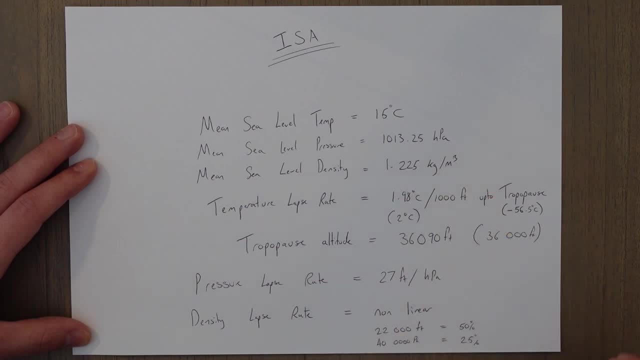 meter cubed. so it's not exact but it's close enough. And if we have deviations from the ISA atmosphere, it's usually defined as a temperature deviation, so you would say an ISA deviation of plus or minus degrees. If at sea level it was 12 degrees, that would be a ISA minus 3 kind of day. Another quick example of ISA deviations. at an altitude of 30,000 feet, the temperature is minus 37, what is the ISA deviation? So normally, you've got to well, basically you've got to find out the normal temperature at 30,000 feet in. 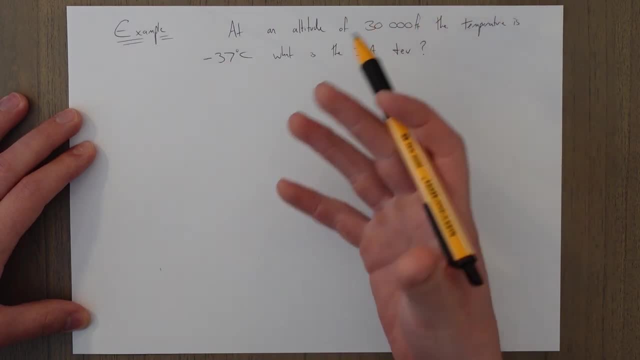 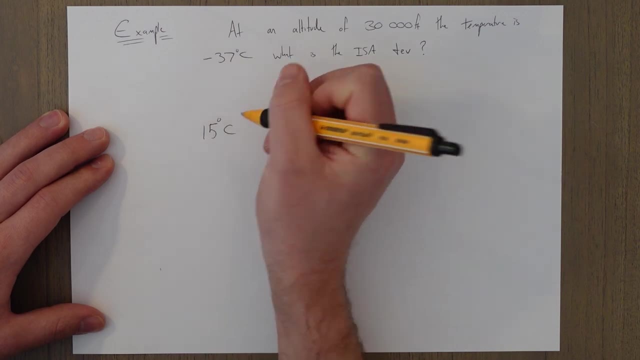 the ISA atmosphere. compare it to this and find out what the deviation is. We can do this very simply. we've got 15 degrees Celsius, which is standard at sea level. We're at 30,000 feet. we're going to drop by the. 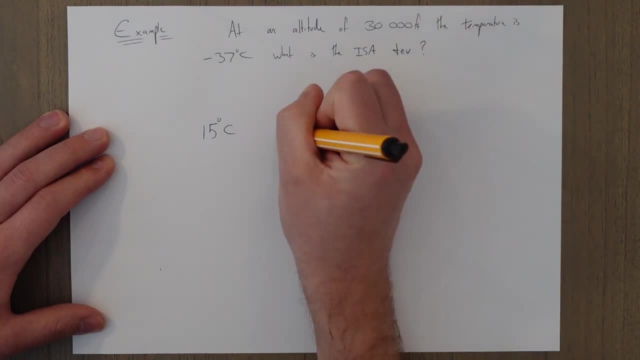 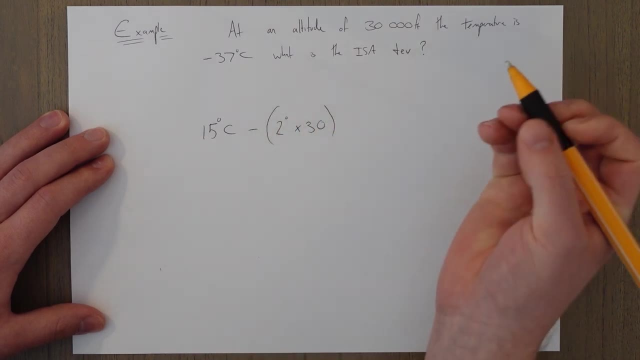 temperature lapse rate, which is 2 degrees per thousand feet. so that's 2 degrees per thousand feet. there's 30 of them, So we know that it reduces. so it's gonna be 15 minus 60 and that's gonna equal minus 45 degrees Celsius in ISA.